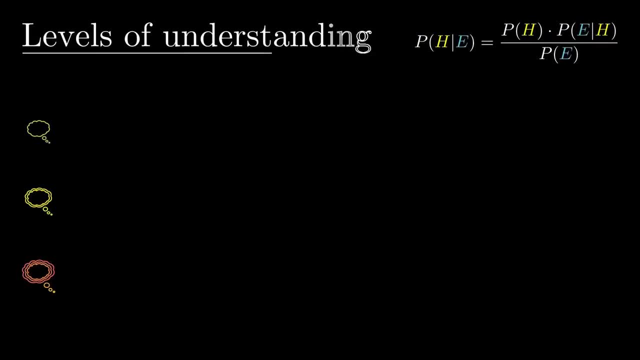 So it's a formula worth understanding, but of course there are multiple different levels of possible understanding. At the simplest, there's just knowing what each one of the parts means, so that you can plug in numbers. Then there's understanding why it's true. 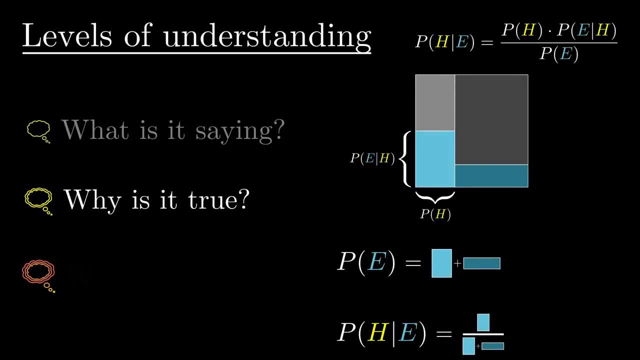 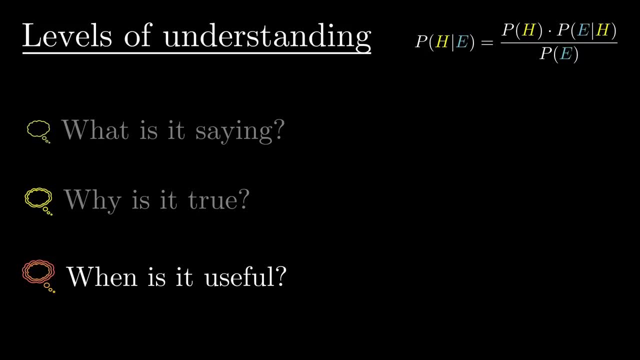 and later I'm going to show you a certain diagram that's helpful for rediscovering this formula on the fly, as needed. But maybe the most important level is being able to recognize when you need to use it. And, with the goal of gaining a deeper understanding, you and I are going to tackle these in reverse. 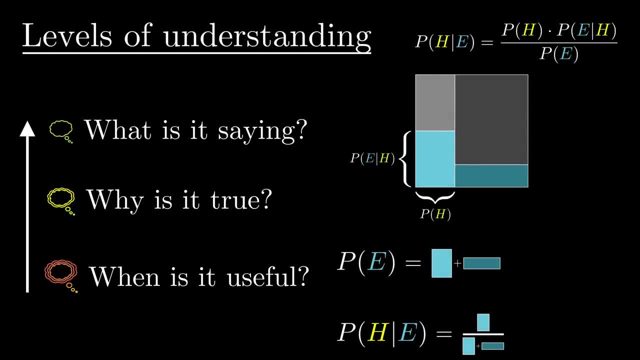 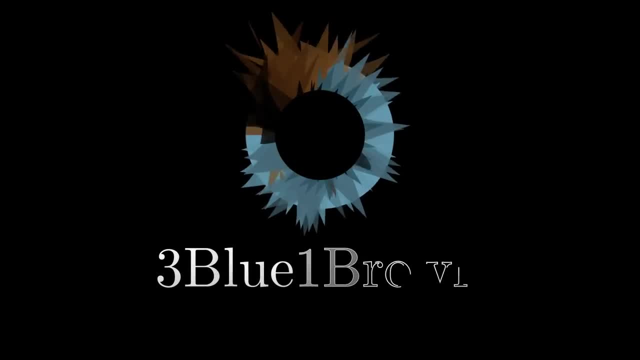 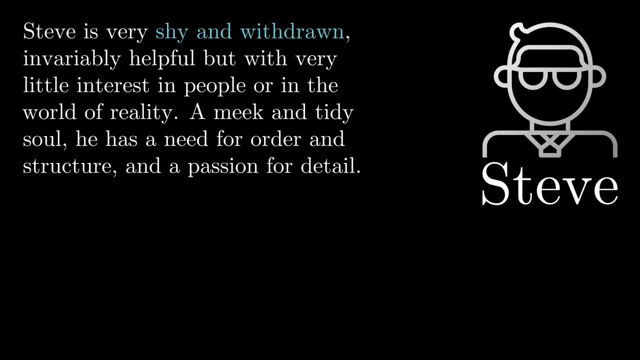 order. So, before dissecting the formula or explaining the visual that makes it obvious, I'd like to tell you about a man named Steve. Listen carefully now. Steve is very shy and withdrawn, invariably helpful, but with very little interest in people or the world of reality. A meek and tidy soul, he has a need for order and structure and 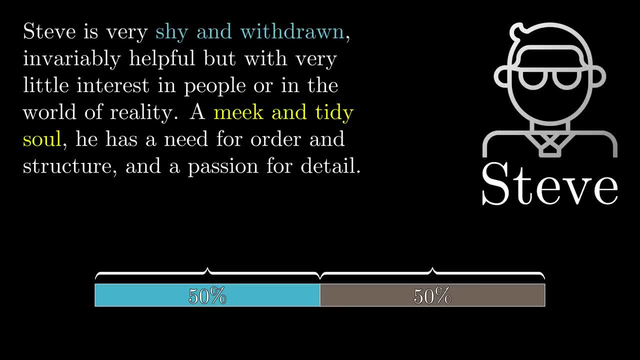 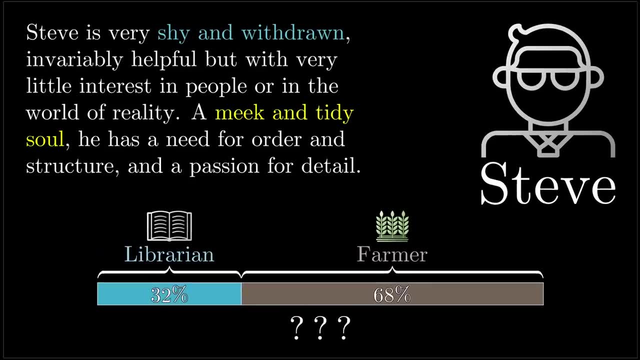 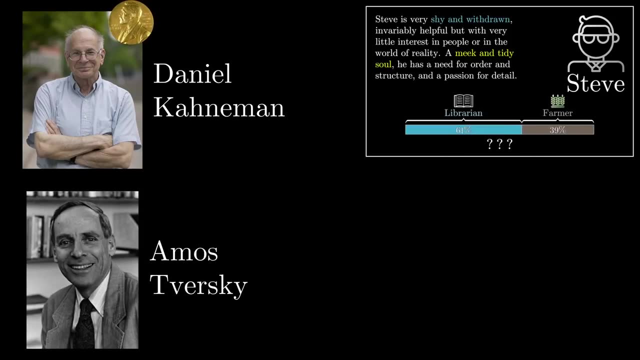 a passion for detail. Which of the following do you find more likely: Steve as a librarian or Steve as a farmer? Some of you may recognize this as an example from a study conducted by the two psychologists Daniel Kahneman and Amos Tversky. Their work was a big deal. It won a Nobel Prize and 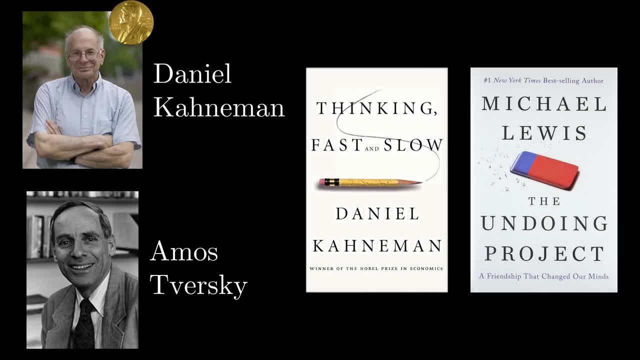 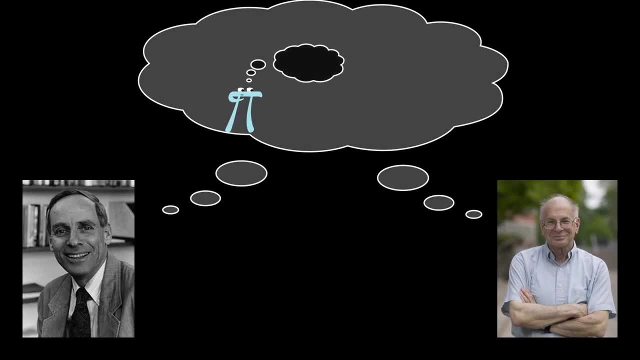 it's been popularized many times over in books like Kahneman's Thinking Fast and Slow or Michael Lewis's The Undoing Project. What they researched was human judgments, with a frequent focus on when these judgments irrationally contradict what the laws of probability say. 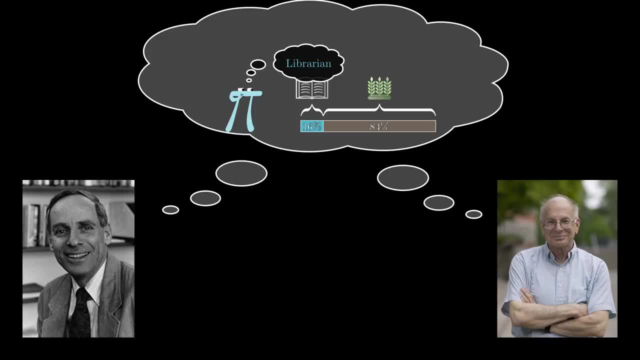 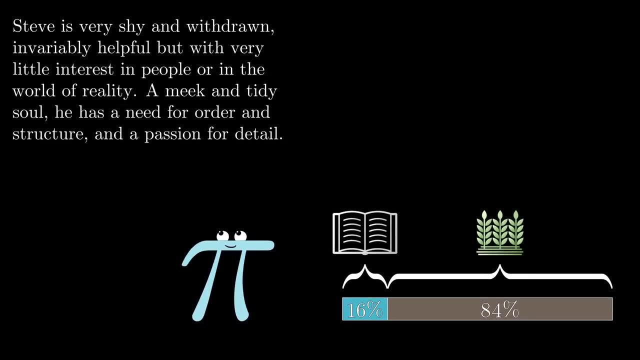 The example with Steve, our maybe-librarian, maybe-farmer, illustrates one specific type of irrationality, Or maybe I should say alleged irrationality. There are people who debate the conclusion here, but more on all of that later on. According to Kahneman and Tversky, after people are given this description of Steve as a meek, 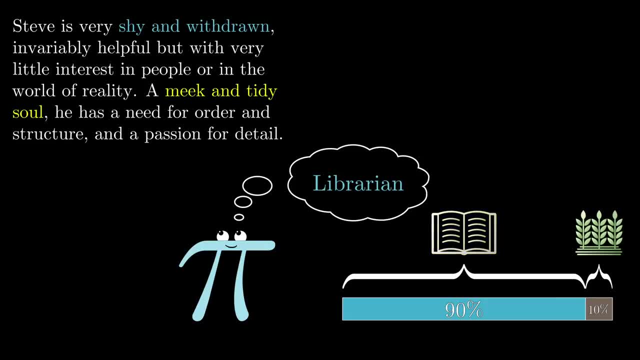 and tidy soul, most say that he's more likely to be a librarian. After all, these traits line up better with the stereotypical view of a librarian than a farmer, And according to Kahneman and Tversky this is irrational. The point is not whether people hold correct or biased views about the personalities of 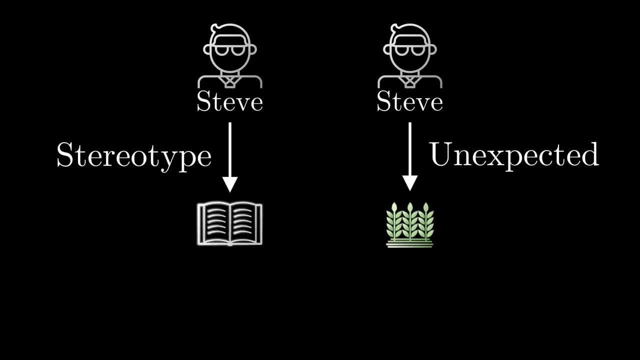 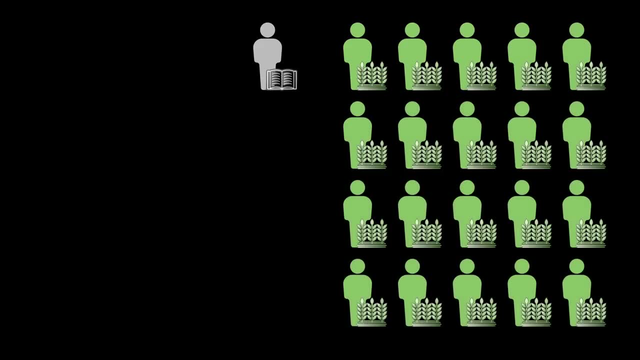 librarians and farmers. It's that almost nobody thinks to incorporate information about the ratio of farmers to librarians in their judgments. In their paper, Kahneman and Tversky said that in the US that ratio is about 20 to 1.. 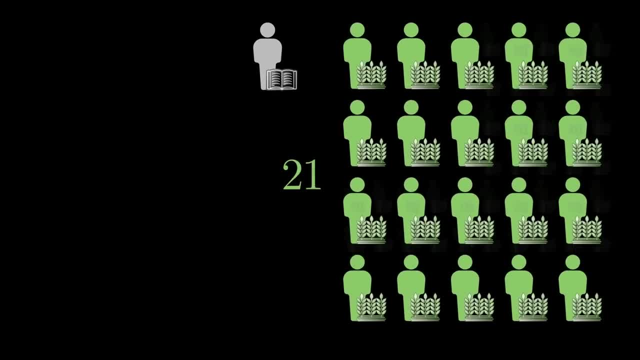 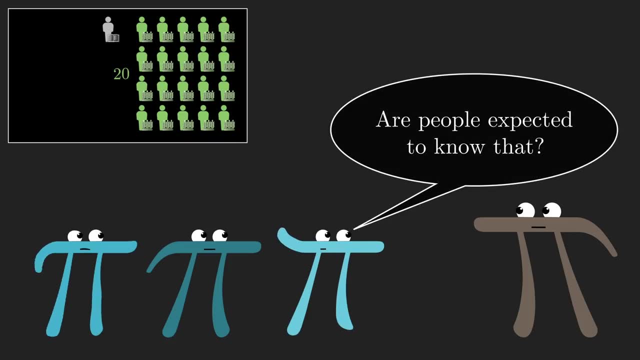 The numbers that I could find today put that actually much higher, but let's stick with the 20 to 1 number, since it's a little easier to illustrate and it proves the point just as well. To be clear, anyone who has asked this question is not expected to have perfect information. 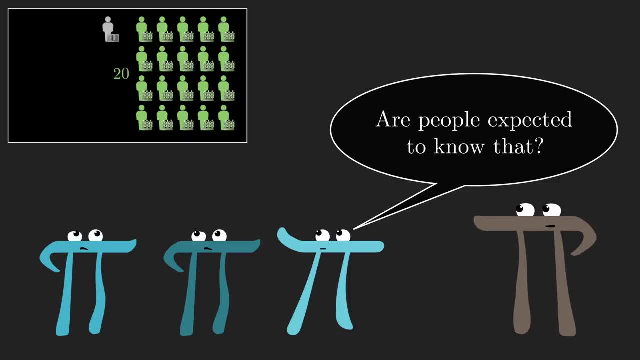 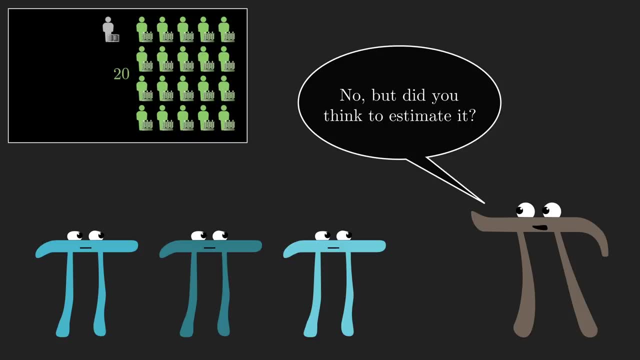 about the actual statistics of farmers and librarians and their personality traits. But the question is whether people even think to consider that ratio enough to at least make a rough estimate. Rationality is not about knowing facts. it's about recognizing which facts are relevant. 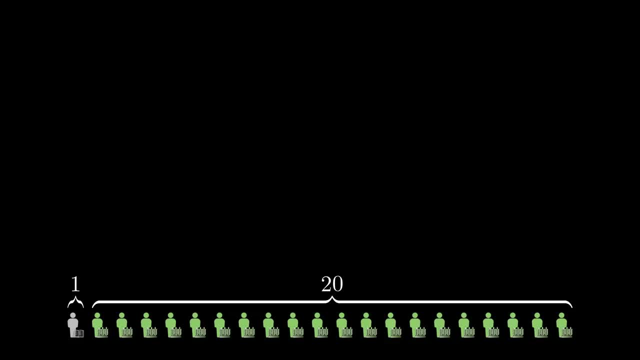 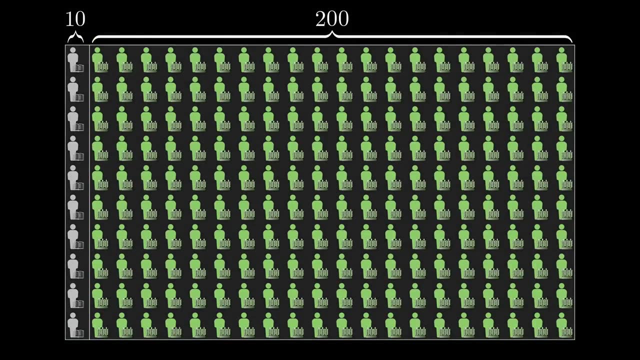 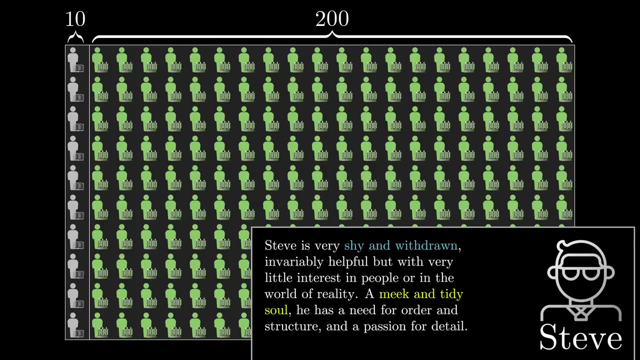 Now, if you do think to make that estimate, there's a pretty simple way to reason about the question, Which spoiler alert involves all of the essential reasoning behind Bayes' theorem. You might start by picturing a representative sample of farmers and librarians, say, 200 farmers and 10 librarians. Then, when you hear of this meek and tidy 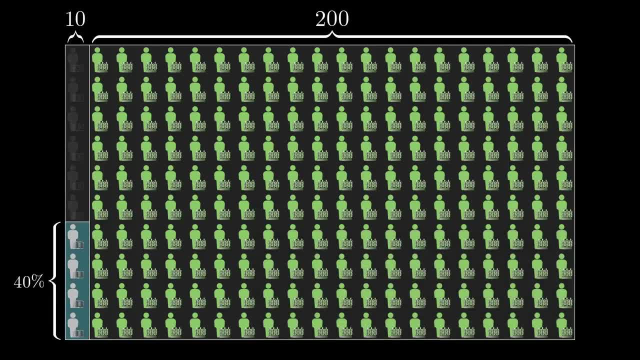 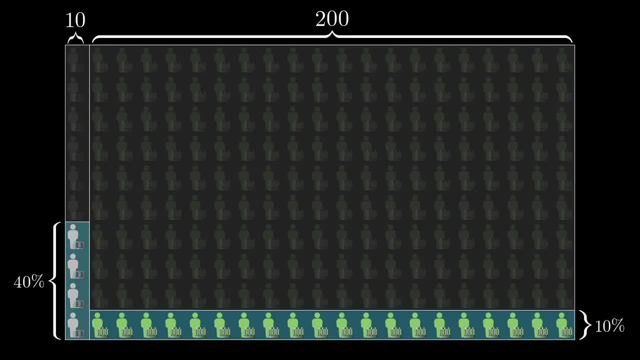 soul description. let's say that your gut instinct is that 40% of librarians would fit that description and that 10% of farmers would. If those are your estimates, it would mean that from your sample, you would expect about 4 librarians to fit the description. 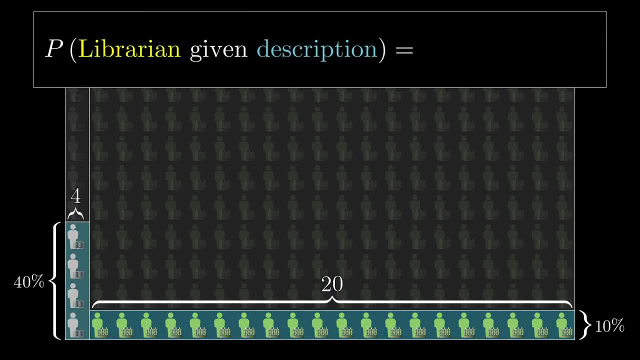 and about 20 farmers to fit that description. So The probability that a random person among those who fit this description is a librarian is 4 out of 24, or 16.7%. So even if you think that a librarian is 4 times as likely as a farmer to fit this description, 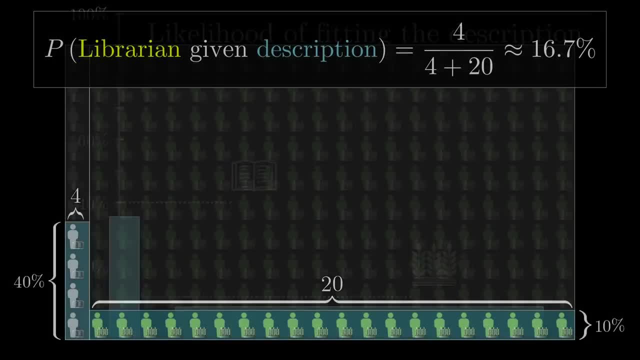 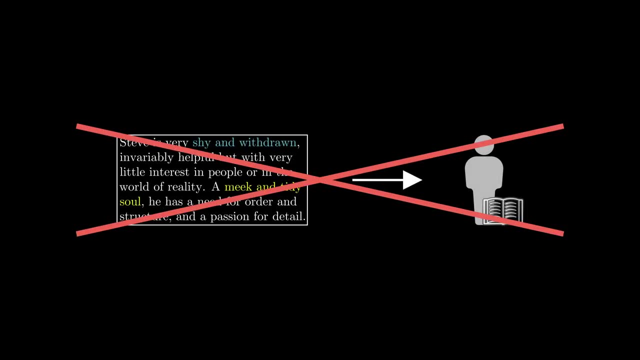 that's not enough to overcome the fact that there are way more farmers. The upshot- and this is the key mantra underlying Bayes' theorem- is that new evidence does not completely determine your beliefs in a vacuum. It should update prior beliefs. 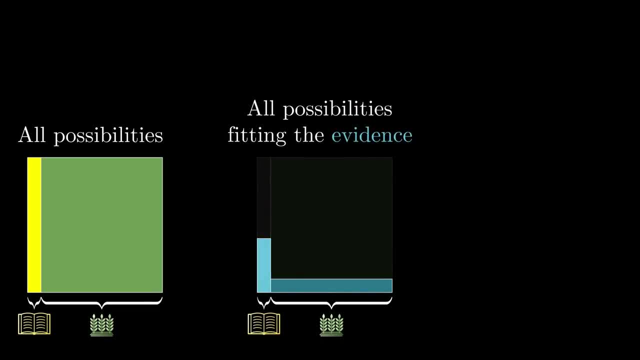 If this line of reasoning makes sense to you, the way that seeing evidence restricts the space of possibilities and the ratio you need to consider after that, then congratulations, you understand the heart of Bayes' theorem. Maybe the numbers you would estimate would. 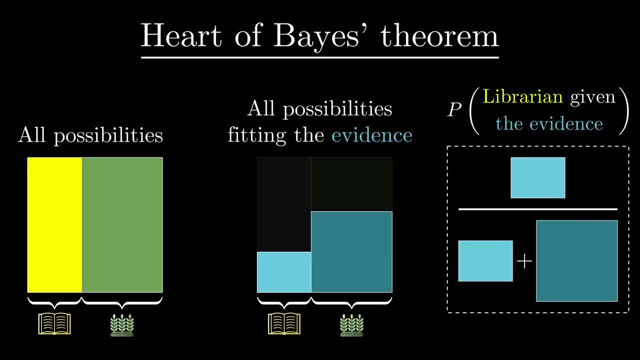 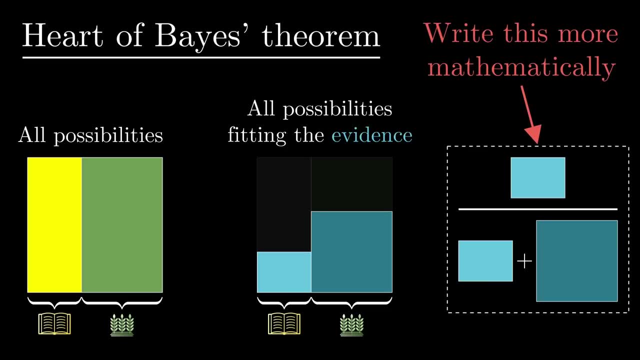 be a little different, but what matters is how you fit the numbers together to update your beliefs based on evidence. Understanding one example is one thing, but see if you can take a minute to generalize everything we just did and write it all down as a formula. 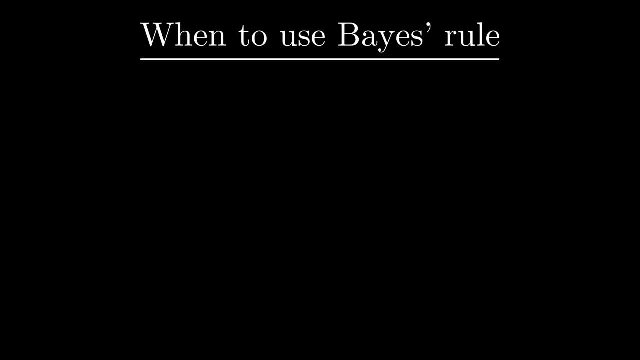 The general situation where Bayes' theorem is relevant is when you have some hypothesis like Steve is a librarian, and you see some new evidence, say this verbal description of Steve as a meek and tidy soul, and you want to know the probability that your hypothesis. 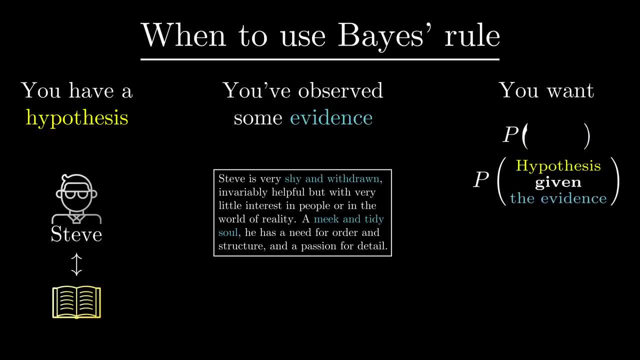 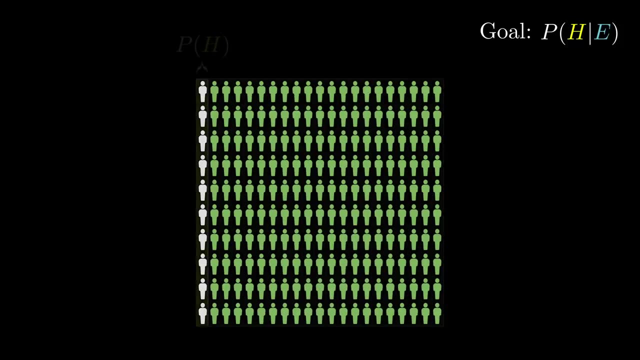 holds, given that the evidence is true. In the standard notation this vertical bar means, given that, as in, we are restricting our view only to the possibilities where the evidence holds. This is the first relevant number we used. It was the probability that the hypothesis 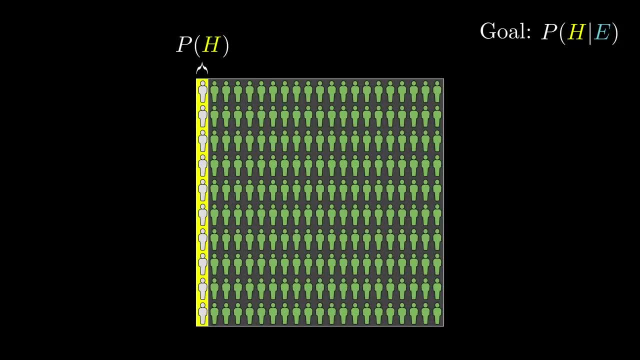 holds before considering any of that new evidence. In our example, that was 1 out of 21, and it came from considering the ratio of librarians to farmers in the general population. This number is known as the prior. After that we need to consider the proportion of librarians that fit this description, the 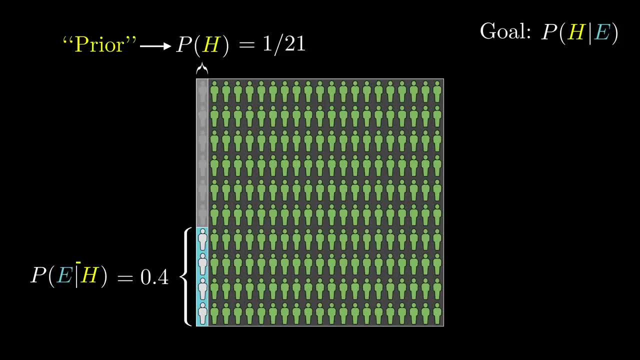 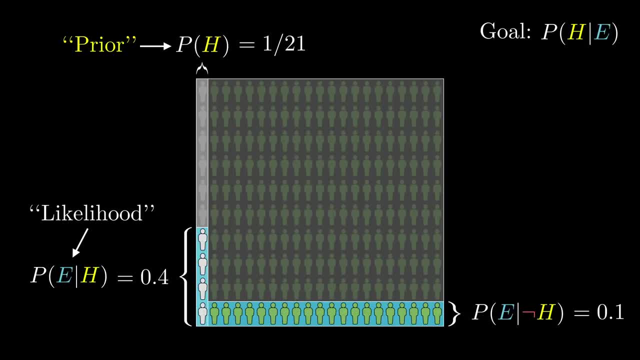 this vertical bar. it means we're talking about the probability that we would see the evidence given that the hypothesis is true. Again, when you see this vertical bar, it means we're talking about the probability that we would see the evidence given that the hypothesis is true. Again, when you see this vertical bar, it means we're talking. about the probability that we would see the evidence, given that the hypothesis is true. Again, when you see this vertical bar, it means we're talking about the probability that we would see the evidence, given that the hypothesis is true. Again, when you see, 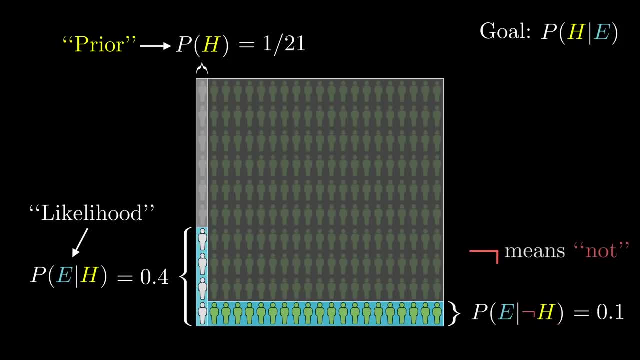 this vertical bar. it means we're talking about the probability that we would see the evidence given that the hypothesis is true. Again, when you see this vertical bar, it means we're talking about the probability that we would see the evidence given that the hypothesis is true. Again, when you see this vertical bar, it means we're talking. about the probability that we would see the evidence, given that the hypothesis is true. Again, when you see this vertical bar, it means we're talking about the probability that we would see the evidence, given that the hypothesis is true. Again, when you see, 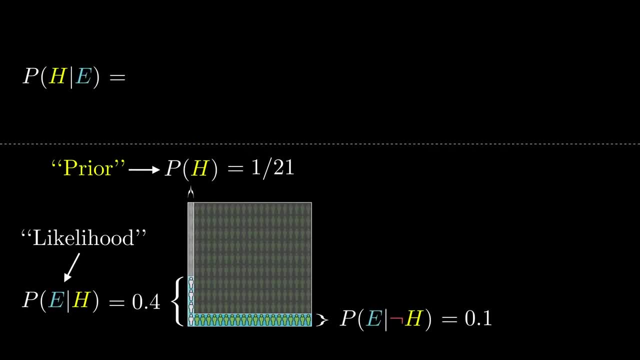 this vertical bar. it means we're talking about the probability that we would see the evidence given that the hypothesis is true. Again, when you see this vertical bar, it means we're talking about the probability that we would see the evidence given that the hypothesis is true. Again, when you see this vertical bar, it means we're talking. about the probability that we would see the evidence, given that the hypothesis is true. Again, when you see this vertical bar, it means we're talking about the probability that we would see the evidence, given that the hypothesis is true. Again, when you see, 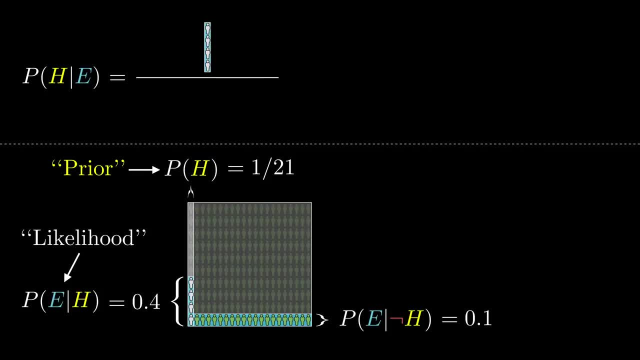 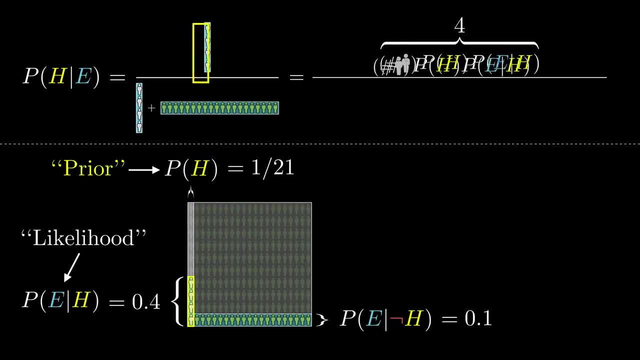 this vertical bar. it means we're talking about the probability that we would see the evidence given that the hypothesis is true. Again, when you see this vertical bar, it means we're talking about the probability that we would see the evidence given that the hypothesis is true. Again, when you see this vertical bar, it means we're talking. about the probability that we would see the evidence, given that the hypothesis is true. Again, when you see this vertical bar, it means we're talking about the probability that we would see the evidence, given that the hypothesis is true. Again, when you see, 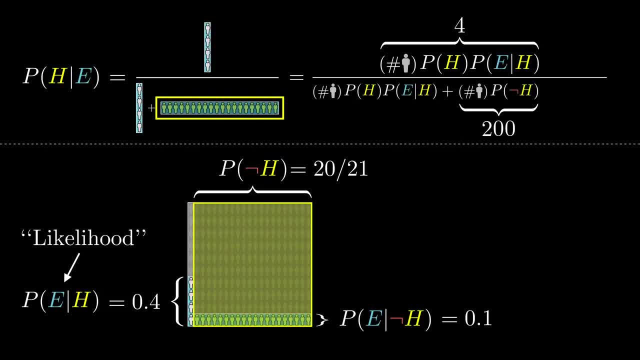 this vertical bar. it means we're talking about the probability that we would see the evidence given that the hypothesis is true. Again, when you see this vertical bar, it means we're talking about the probability that we would see the evidence given that the hypothesis is true. Again, when you see this vertical bar, it means we're talking. about the probability that we would see the evidence, given that the hypothesis is true. Again, when you see this vertical bar, it means we're talking about the probability that we would see the evidence, given that the hypothesis is true. Again, when you see, 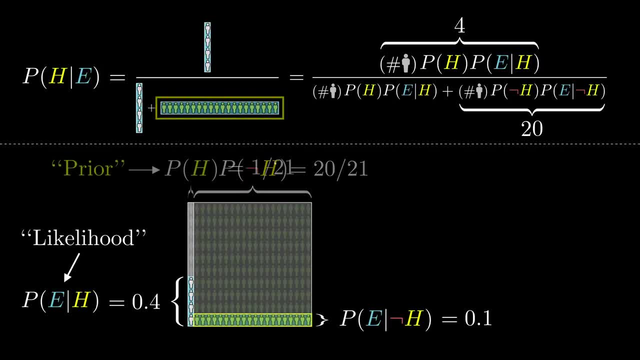 this vertical bar. it means we're talking about the probability that we would see the evidence given that the hypothesis is true. Again, when you see this vertical bar, it means we're talking about the probability that we would see the evidence given that the hypothesis is true. Again, when you see this vertical bar, it means we're talking. about the probability that we would see the evidence, given that the hypothesis is true. Again, when you see this vertical bar, it means we're talking about the probability that we would see the evidence, given that the hypothesis is true. Again, when you see, 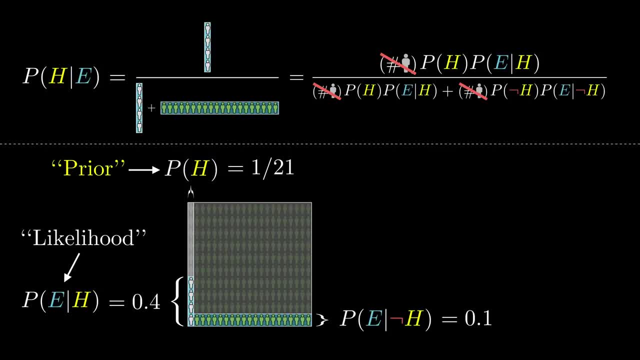 this vertical bar. it means we're talking about the probability that we would see the evidence given that the hypothesis is true. Again, when you see this vertical bar, it means we're talking about the probability that we would see the evidence given that the hypothesis is true. Again, when you see this vertical bar, it means we're talking. about the probability that we would see the evidence, given that the hypothesis is true. Again, when you see this vertical bar, it means we're talking about the probability that we would see the evidence, given that the hypothesis is true. Again, when you see, 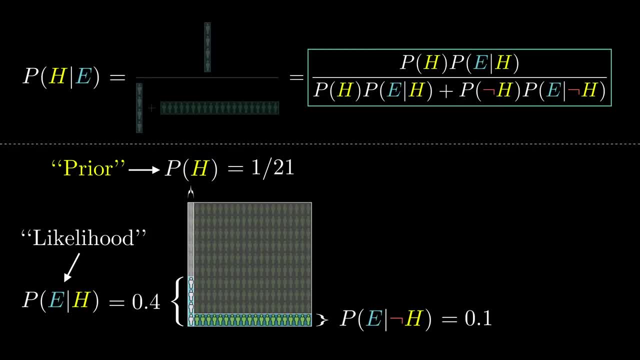 this vertical bar. it means we're talking about the probability that we would see the evidence given that the hypothesis is true. Again, when you see this vertical bar, it means we're talking about the probability that we would see the evidence given that the hypothesis is true. Again, when you see this vertical bar, it means we're talking. about the probability that we would see the evidence, given that the hypothesis is true. Again, when you see this vertical bar, it means we're talking about the probability that we would see the evidence, given that the hypothesis is true. Again, when you see, 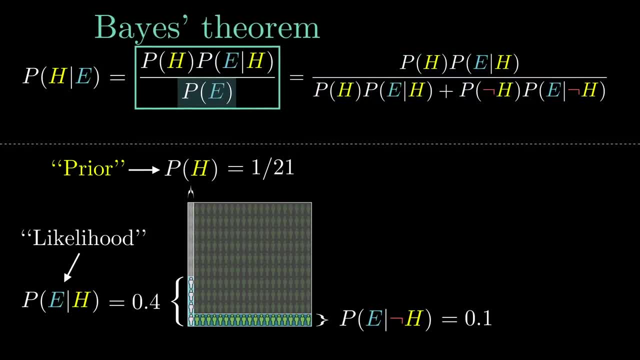 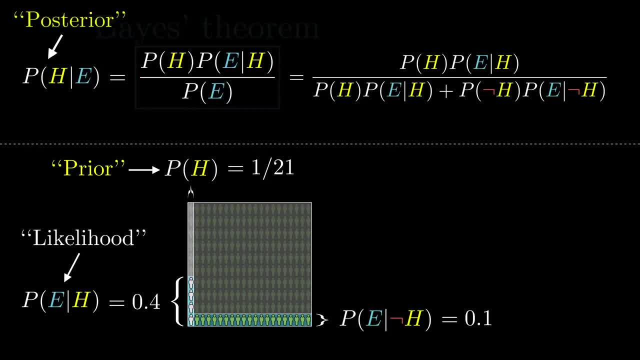 this vertical bar. it means we're talking about the probability that we would see the evidence given that the hypothesis is true. Again, when you see this vertical bar, it means we're talking about the probability that we would see the evidence given that the hypothesis is true. Again, when you see this vertical bar, it means we're talking. about the probability that we would see the evidence, given that the hypothesis is true. Again, when you see this vertical bar, it means we're talking about the probability that we would see the evidence, given that the hypothesis is true. Again, when you see, 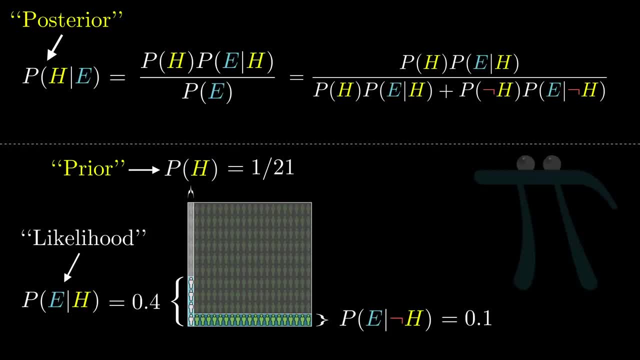 this vertical bar. it means we're talking about the probability that we would see the evidence given that the hypothesis is true. Again, when you see this vertical bar, it means we're talking about the probability that we would see the evidence given that the hypothesis is true. Again, when you see this vertical bar, it means we're talking. about the probability that we would see the evidence, given that the hypothesis is true. Again, when you see this vertical bar, it means we're talking about the probability that we would see the evidence, given that the hypothesis is true. Again, when you see, 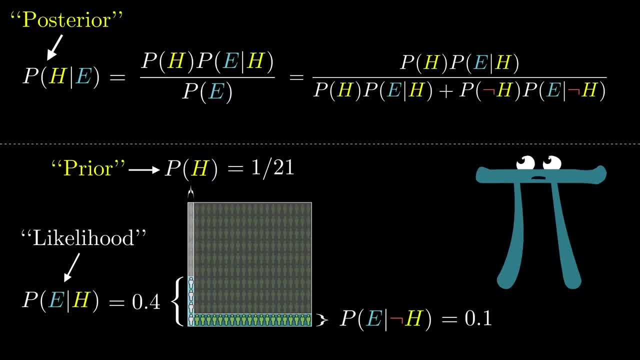 this vertical bar. it means we're talking about the probability that we would see the evidence given that the hypothesis is true. Again, when you see this vertical bar, it means we're talking about the probability that we would see the evidence given that the hypothesis is true. Again, when you see this vertical bar, it means we're talking. about the probability that we would see the evidence, given that the hypothesis is true. Again, when you see this vertical bar, it means we're talking about the probability that we would see the evidence, given that the hypothesis is true. Again, when you see, 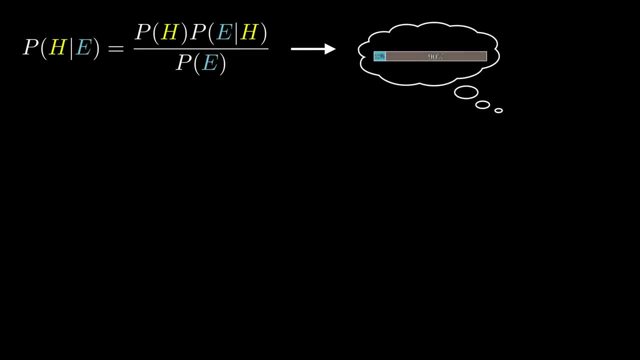 this vertical bar. it means we're talking about the probability that we would see the evidence given that the hypothesis is true. Again, when you see this vertical bar, it means we're talking about the probability that we would see the evidence given that the hypothesis is true. Again, when you see this vertical bar, it means we're talking. about the probability that we would see the evidence, given that the hypothesis is true. Again, when you see this vertical bar, it means we're talking about the probability that we would see the evidence, given that the hypothesis is true. Again, when you see, 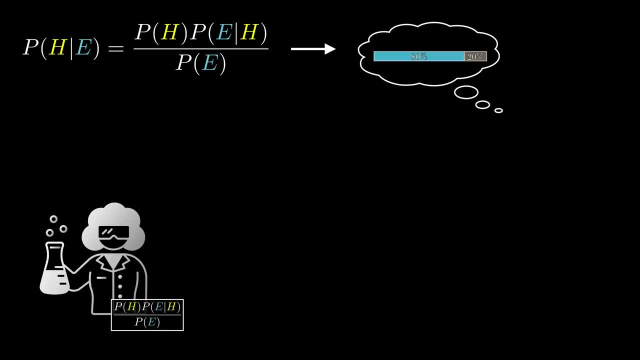 this vertical bar. it means we're talking about the probability that we would see the evidence given that the hypothesis is true. Again, when you see this vertical bar, it means we're talking about the probability that we would see the evidence given that the hypothesis is true. Again, when you see this vertical bar, it means we're talking. about the probability that we would see the evidence, given that the hypothesis is true. Again, when you see this vertical bar, it means we're talking about the probability that we would see the evidence, given that the hypothesis is true. Again, when you see, 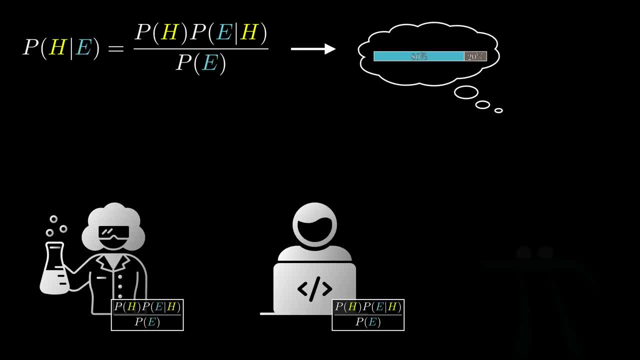 this vertical bar. it means we're talking about the probability that we would see the evidence given that the hypothesis is true. Again, when you see this vertical bar, it means we're talking about the probability that we would see the evidence given that the hypothesis is true. Again, when you see this vertical bar, it means we're talking. about the probability that we would see the evidence, given that the hypothesis is true. Again, when you see this vertical bar, it means we're talking about the probability that we would see the evidence, given that the hypothesis is true. Again, when you see, 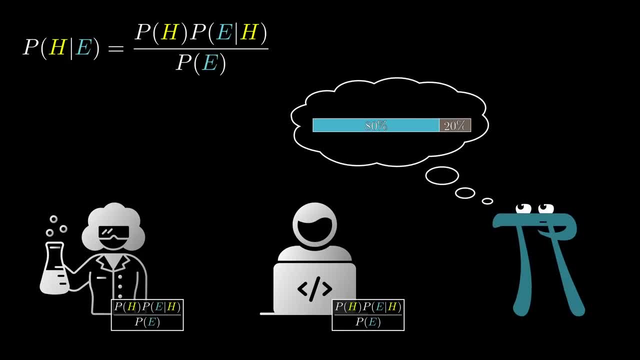 this vertical bar. it means we're talking about the probability that we would see the evidence given that the hypothesis is true. Again, when you see this vertical bar, it means we're talking about the probability that we would see the evidence given that the hypothesis is true. Again, when you see this vertical bar, it means we're talking. about the probability that we would see the evidence, given that the hypothesis is true. Again, when you see this vertical bar, it means we're talking about the probability that we would see the evidence, given that the hypothesis is true. Again, when you see, 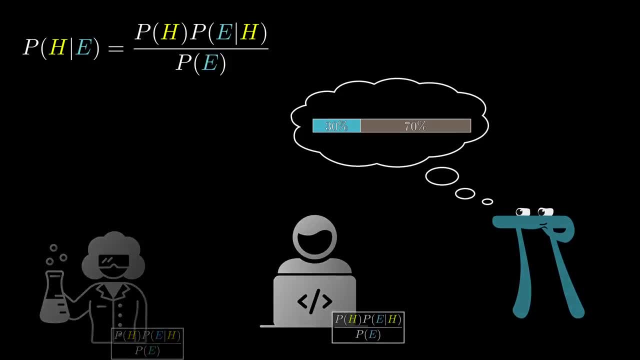 this vertical bar. it means we're talking about the probability that we would see the evidence given that the hypothesis is true. Again, when you see this vertical bar, it means we're talking about the probability that we would see the evidence given that the hypothesis is true. Again, when you see this vertical bar, it means we're talking. about the probability that we would see the evidence, given that the hypothesis is true. Again, when you see this vertical bar, it means we're talking about the probability that we would see the evidence, given that the hypothesis is true. Again, when you see, 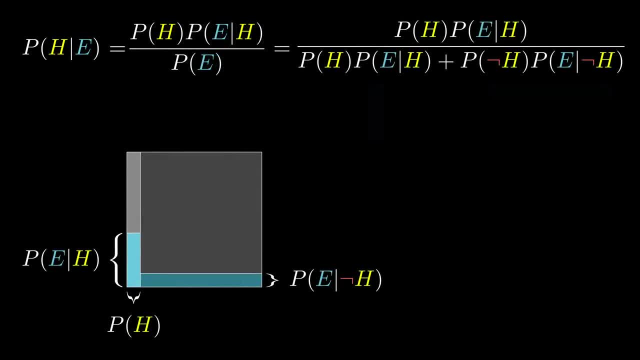 this vertical bar. it means we're talking about the probability that we would see the evidence given that the hypothesis is true. Again, when you see this vertical bar, it means we're talking about the probability that we would see the evidence given that the hypothesis is true. Again, when you see this vertical bar, it means we're talking. about the probability that we would see the evidence, given that the hypothesis is true. Again, when you see this vertical bar, it means we're talking about the probability that we would see the evidence, given that the hypothesis is true. Again, when you see, 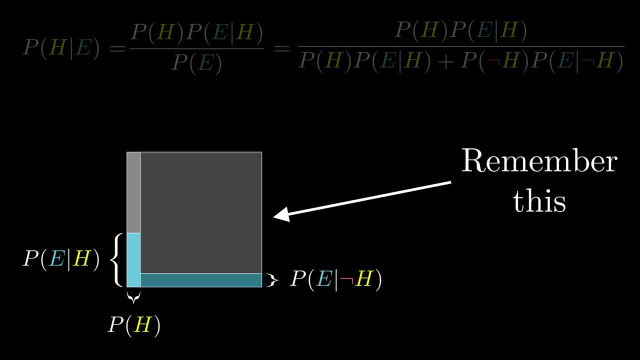 this vertical bar. it means we're talking about the probability that we would see the evidence given that the hypothesis is true. Again, when you see this vertical bar, it means we're talking about the probability that we would see the evidence given that the hypothesis is true. Again, when you see this vertical bar, it means we're talking. about the probability that we would see the evidence, given that the hypothesis is true. Again, when you see this vertical bar, it means we're talking about the probability that we would see the evidence, given that the hypothesis is true. Again, when you see, 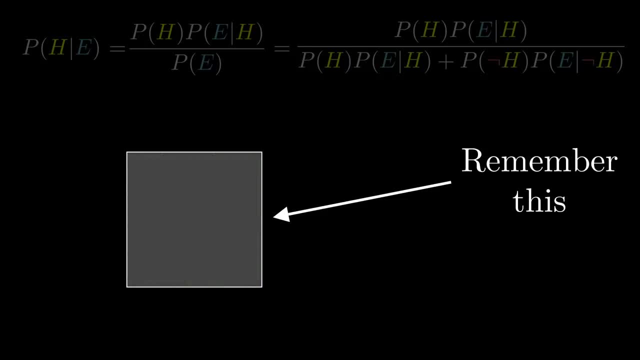 this vertical bar. it means we're talking about the probability that we would see the evidence given that the hypothesis is true. Again, when you see this vertical bar, it means we're talking about the probability that we would see the evidence given that the hypothesis is true. Again, when you see this vertical bar, it means we're talking. about the probability that we would see the evidence, given that the hypothesis is true. Again, when you see this vertical bar, it means we're talking about the probability that we would see the evidence, given that the hypothesis is true. Again, when you see, 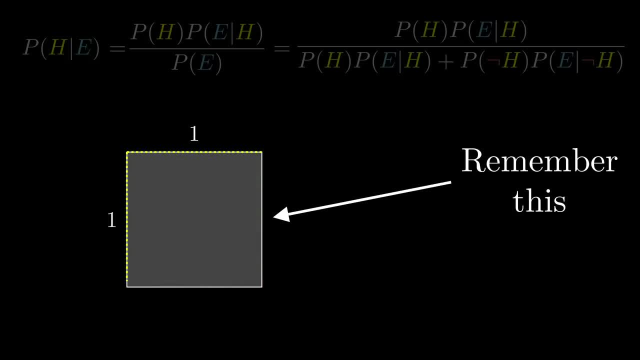 this vertical bar. it means we're talking about the probability that we would see the evidence given that the hypothesis is true. Again, when you see this vertical bar, it means we're talking about the probability that we would see the evidence given that the hypothesis is true. Again, when you see this vertical bar, it means we're talking. about the probability that we would see the evidence, given that the hypothesis is true. Again, when you see this vertical bar, it means we're talking about the probability that we would see the evidence, given that the hypothesis is true. Again, when you see, 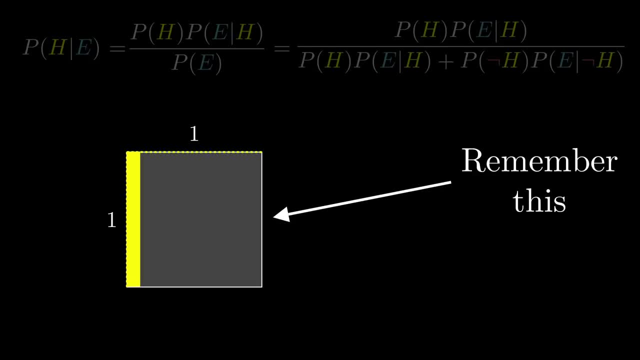 this vertical bar. it means we're talking about the probability that we would see the evidence given that the hypothesis is true. Again, when you see this vertical bar, it means we're talking about the probability that we would see the evidence given that the hypothesis is true. Again, when you see this vertical bar, it means we're talking. about the probability that we would see the evidence, given that the hypothesis is true. Again, when you see this vertical bar, it means we're talking about the probability that we would see the evidence, given that the hypothesis is true. Again, when you see, 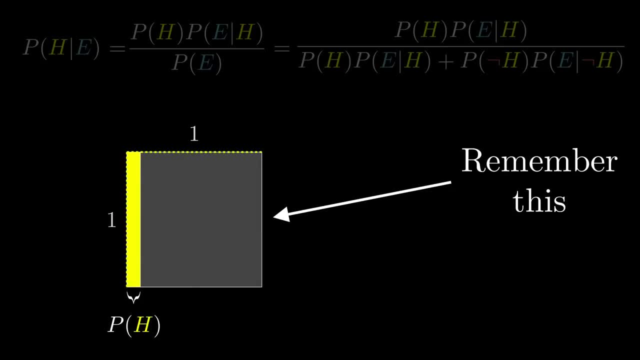 this vertical bar. it means we're talking about the probability that we would see the evidence given that the hypothesis is true. Again, when you see this vertical bar, it means we're talking about the probability that we would see the evidence given that the hypothesis is true. Again, when you see this vertical bar, it means we're talking. about the probability that we would see the evidence, given that the hypothesis is true. Again, when you see this vertical bar, it means we're talking about the probability that we would see the evidence, given that the hypothesis is true. Again, when you see, 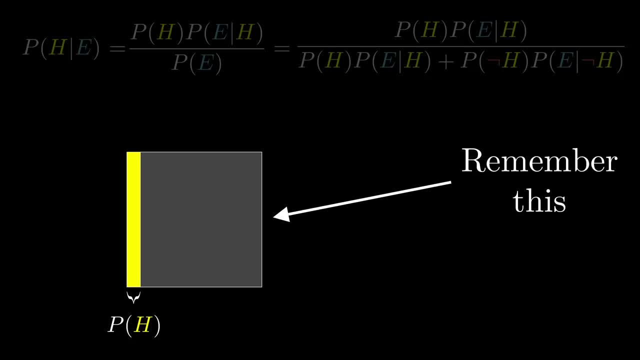 this vertical bar. it means we're talking about the probability that we would see the evidence given that the hypothesis is true. Again, when you see this vertical bar, it means we're talking about the probability that we would see the evidence given that the hypothesis is true. Again, when you see this vertical bar, it means we're talking. about the probability that we would see the evidence, given that the hypothesis is true. Again, when you see this vertical bar, it means we're talking about the probability that we would see the evidence, given that the hypothesis is true. Again, when you see, 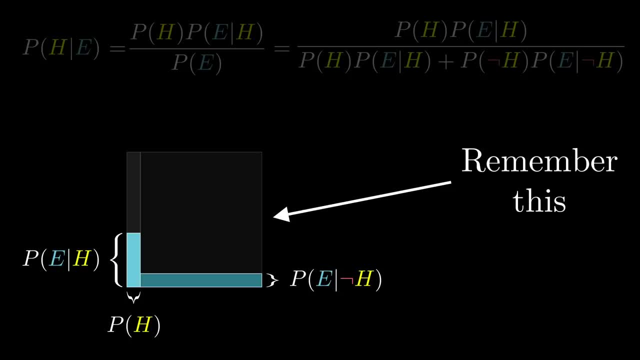 this vertical bar. it means we're talking about the probability that we would see the evidence given that the hypothesis is true. Again, when you see this vertical bar, it means we're talking about the probability that we would see the evidence given that the hypothesis is true. Again, when you see this vertical bar, it means we're talking. about the probability that we would see the evidence, given that the hypothesis is true. Again, when you see this vertical bar, it means we're talking about the probability that we would see the evidence, given that the hypothesis is true. Again, when you see, 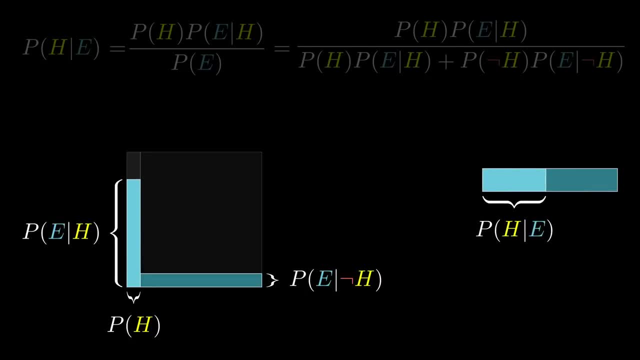 this vertical bar. it means we're talking about the probability that we would see the evidence given that the hypothesis is true. Again, when you see this vertical bar, it means we're talking about the probability that we would see the evidence given that the hypothesis is true. Again, when you see this vertical bar, it means we're talking. about the probability that we would see the evidence, given that the hypothesis is true. Again, when you see this vertical bar, it means we're talking about the probability that we would see the evidence, given that the hypothesis is true. Again, when you see, 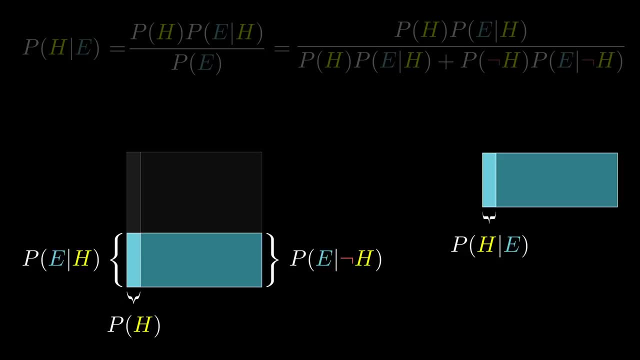 this vertical bar. it means we're talking about the probability that we would see the evidence given that the hypothesis is true. Again, when you see this vertical bar, it means we're talking about the probability that we would see the evidence given that the hypothesis is true. Again, when you see this vertical bar, it means we're talking. about the probability that we would see the evidence, given that the hypothesis is true. Again, when you see this vertical bar, it means we're talking about the probability that we would see the evidence, given that the hypothesis is true. Again, when you see, 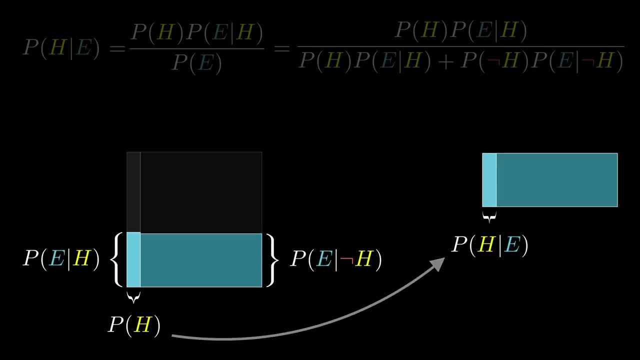 this vertical bar. it means we're talking about the probability that we would see the evidence given that the hypothesis is true. Again, when you see this vertical bar, it means we're talking about the probability that we would see the evidence given that the hypothesis is true. Again, when you see this vertical bar, it means we're talking. about the probability that we would see the evidence, given that the hypothesis is true. Again, when you see this vertical bar, it means we're talking about the probability that we would see the evidence, given that the hypothesis is true. Again, when you see, 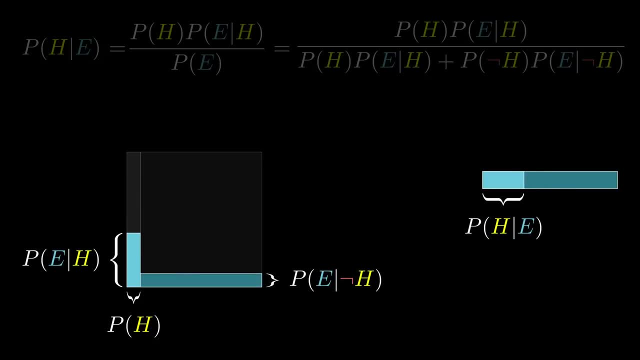 this vertical bar. it means we're talking about the probability that we would see the evidence given that the hypothesis is true. Again, when you see this vertical bar, it means we're talking about the probability that we would see the evidence given that the hypothesis is true. Again, when you see this vertical bar, it means we're talking. 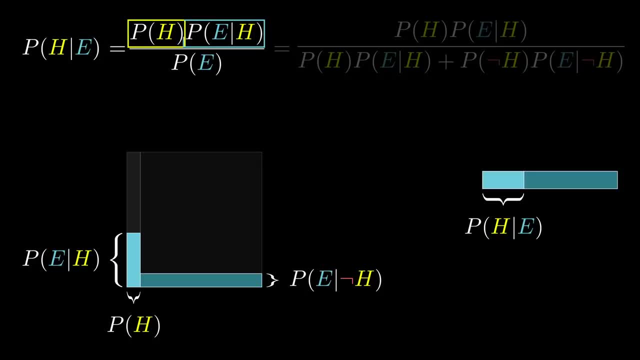 this vertical bar. it means we're talking about the probability that we would see the evidence given that the hypothesis is true. Again, when you see this vertical bar, it means we're talking about the probability that we would see the evidence given that the hypothesis is true. Again, when you see this vertical bar, it means we're talking. about the probability that we would see the evidence, given that the hypothesis is true. Again, when you see this vertical bar, it means we're talking about the probability that we would see the evidence, given that the hypothesis is true. Again, when you see, 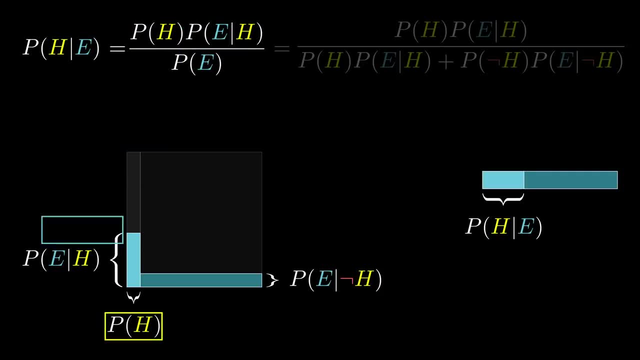 this vertical bar. it means we're talking about the probability that we would see the evidence given that the hypothesis is true. Again, when you see this vertical bar, it means we're talking about the probability that we would see the evidence given that the hypothesis is true. Again, when you see this vertical bar, it means we're talking. about the probability that we would see the evidence, given that the hypothesis is true. Again, when you see this vertical bar, it means we're talking about the probability that we would see the evidence, given that the hypothesis is true. Again, when you see, 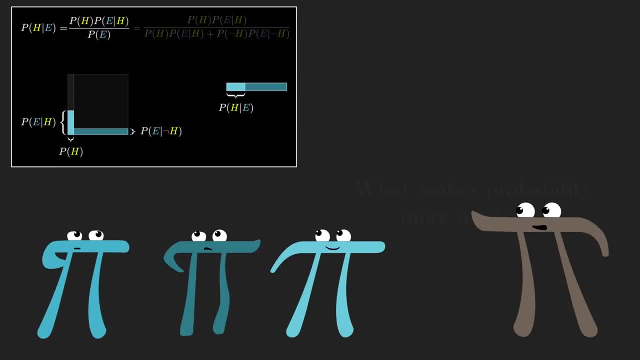 this vertical bar. it means we're talking about the probability that we would see the evidence given that the hypothesis is true. Again, when you see this vertical bar, it means we're talking about the probability that we would see the evidence given that the hypothesis is true. Again, when you see this vertical bar, it means we're talking. about the probability that we would see the evidence, given that the hypothesis is true. Again, when you see this vertical bar, it means we're talking about the probability that we would see the evidence, given that the hypothesis is true. Again, when you see, 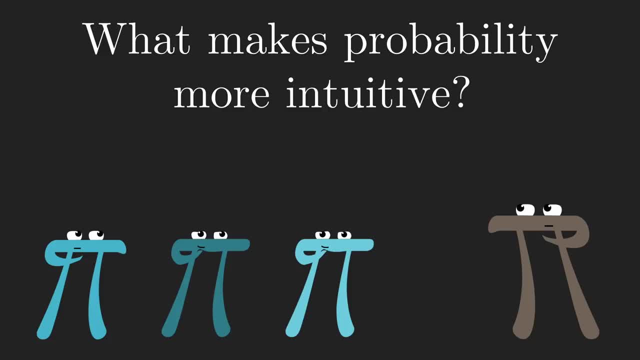 this vertical bar. it means we're talking about the probability that we would see the evidence given that the hypothesis is true. Again, when you see this vertical bar, it means we're talking about the probability that we would see the evidence given that the hypothesis is true. Again, when you see this vertical bar, it means we're talking. about the probability that we would see the evidence, given that the hypothesis is true. Again, when you see this vertical bar, it means we're talking about the probability that we would see the evidence, given that the hypothesis is true. Again, when you see, 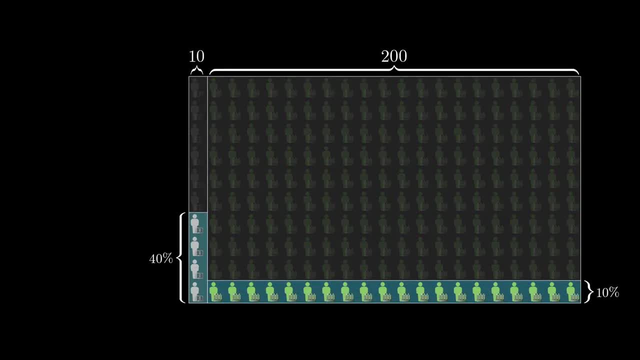 this vertical bar. it means we're talking about the probability that we would see the evidence given that the hypothesis is true. Again, when you see this vertical bar, it means we're talking about the probability that we would see the evidence given that the hypothesis is true. Again, when you see this vertical bar, it means we're talking. about the probability that we would see the evidence, given that the hypothesis is true. Again, when you see this vertical bar, it means we're talking about the probability that we would see the evidence, given that the hypothesis is true. Again, when you see, 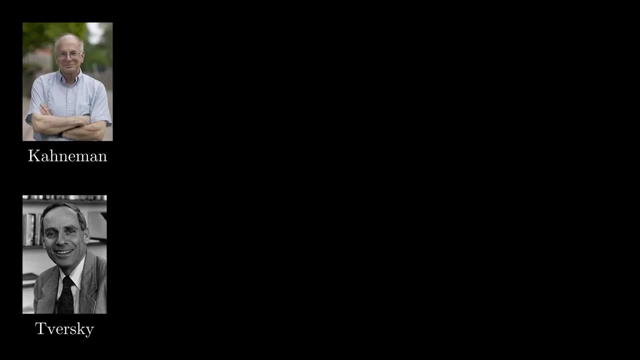 this vertical bar. it means we're talking about the probability that we would see the evidence given that the hypothesis is true. Again, when you see this vertical bar, it means we're talking about the probability that we would see the evidence given that the hypothesis is true. Again, when you see this vertical bar, it means we're talking. about the probability that we would see the evidence, given that the hypothesis is true. Again, when you see this vertical bar, it means we're talking about the probability that we would see the evidence, given that the hypothesis is true. Again, when you see, 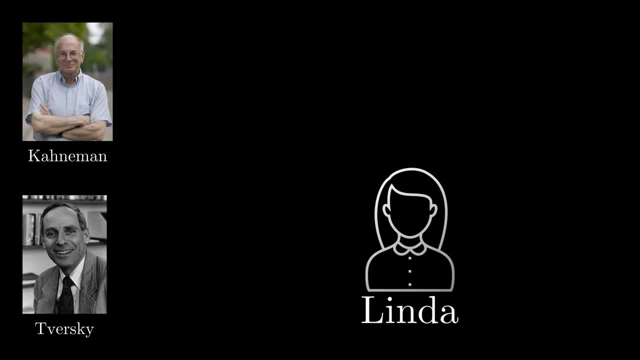 this vertical bar. it means we're talking about the probability that we would see the evidence given that the hypothesis is true. Again, when you see this vertical bar, it means we're talking about the probability that we would see the evidence given that the hypothesis is true. Again, when you see this vertical bar, it means we're talking. about the probability that we would see the evidence, given that the hypothesis is true. Again, when you see this vertical bar, it means we're talking about the probability that we would see the evidence, given that the hypothesis is true. Again, when you see, 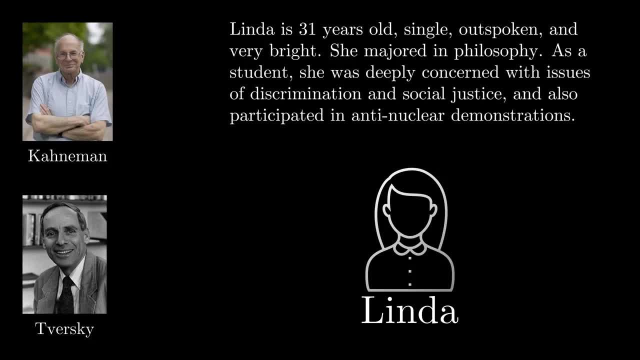 this vertical bar. it means we're talking about the probability that we would see the evidence given that the hypothesis is true. Again, when you see this vertical bar, it means we're talking about the probability that we would see the evidence given that the hypothesis is true. Again, when you see this vertical bar, it means we're talking. about the probability that we would see the evidence, given that the hypothesis is true. Again, when you see this vertical bar, it means we're talking about the probability that we would see the evidence, given that the hypothesis is true. Again, when you see, 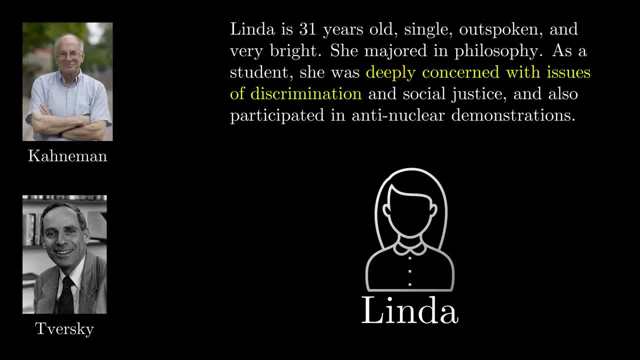 this vertical bar. it means we're talking about the probability that we would see the evidence given that the hypothesis is true. Again, when you see this vertical bar, it means we're talking about the probability that we would see the evidence given that the hypothesis is true. Again, when you see this vertical bar, it means we're talking. about the probability that we would see the evidence, given that the hypothesis is true. Again, when you see this vertical bar, it means we're talking about the probability that we would see the evidence, given that the hypothesis is true. Again, when you see, 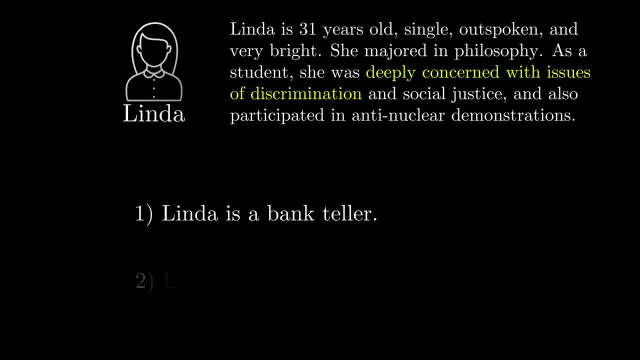 this vertical bar. it means we're talking about the probability that we would see the evidence given that the hypothesis is true. Again, when you see this vertical bar, it means we're talking about the probability that we would see the evidence given that the hypothesis is true. Again, when you see this vertical bar, it means we're talking. about the probability that we would see the evidence, given that the hypothesis is true. Again, when you see this vertical bar, it means we're talking about the probability that we would see the evidence, given that the hypothesis is true. Again, when you see, 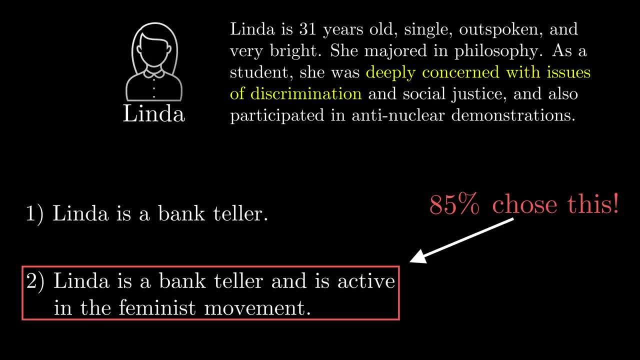 this vertical bar. it means we're talking about the probability that we would see the evidence given that the hypothesis is true. Again, when you see this vertical bar, it means we're talking about the probability that we would see the evidence given that the hypothesis is true. Again, when you see this vertical bar, it means we're talking. about the probability that we would see the evidence, given that the hypothesis is true. Again, when you see this vertical bar, it means we're talking about the probability that we would see the evidence, given that the hypothesis is true. Again, when you see, 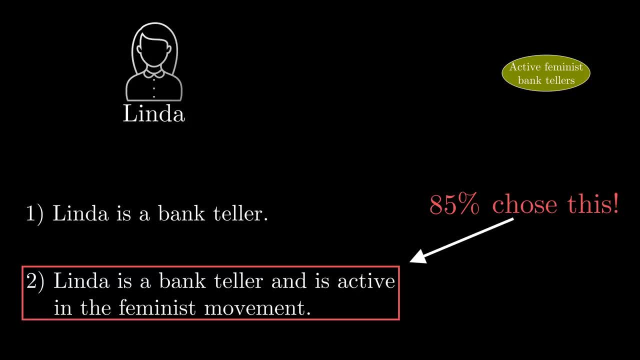 this vertical bar. it means we're talking about the probability that we would see the evidence given that the hypothesis is true. Again, when you see this vertical bar, it means we're talking about the probability that we would see the evidence given that the hypothesis is true. Again, when you see this vertical bar, it means we're talking. 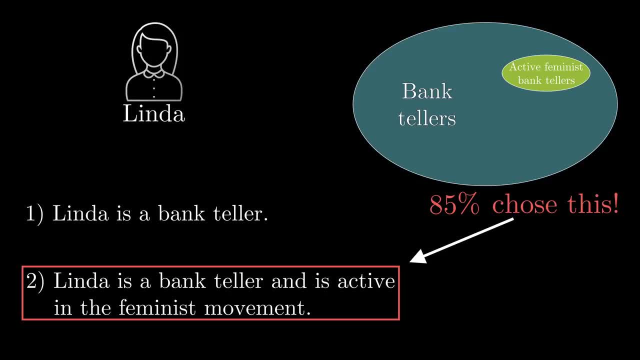 about the probability that we would see the evidence. given that the hypothesis is true, The приб clue answer fits positively Alright, so we're done with this test here. Okay, so we're done with this test here. The trick was to get the right number from Where's thedigitalma? 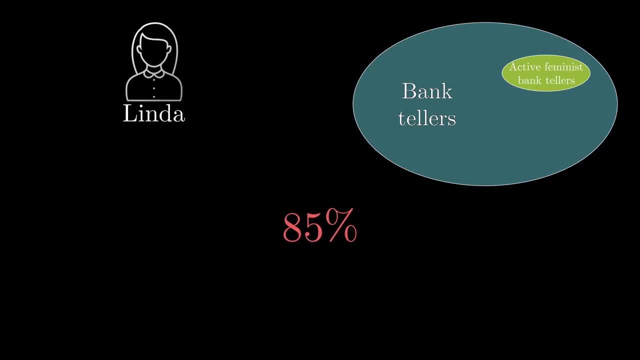 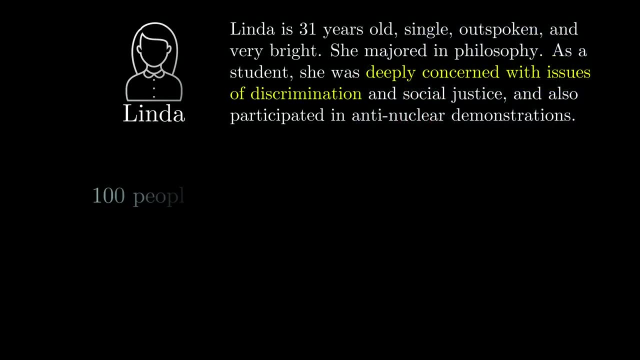 The trick was to get the right number from Where's thedigitalma. We'll give you a half-second break. we'll give you even more time to at least get a hold of the numbers we got from Where's thedigitalma. This took Social Security to Carmichael He. 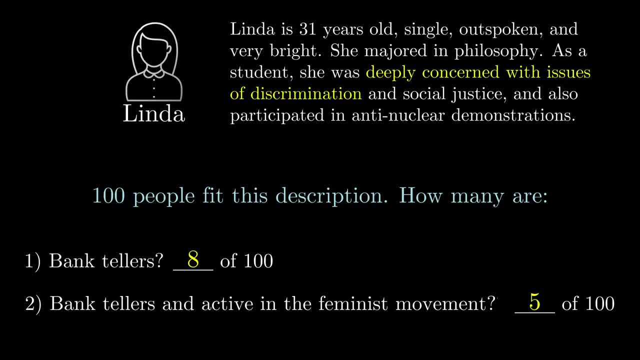 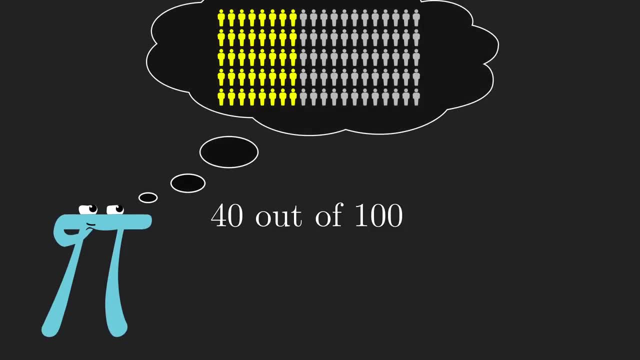 puts Donald Trump inと思います higher number to the first option than to the second. It's weird. somehow phrases like 40 out of 100 kick our intuitions into gear much more effectively than 40%, much less 0.4, and much less. 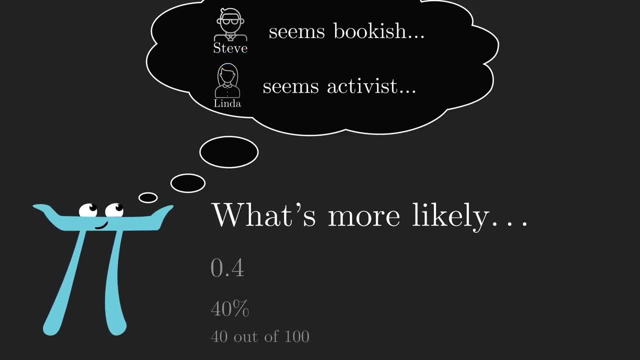 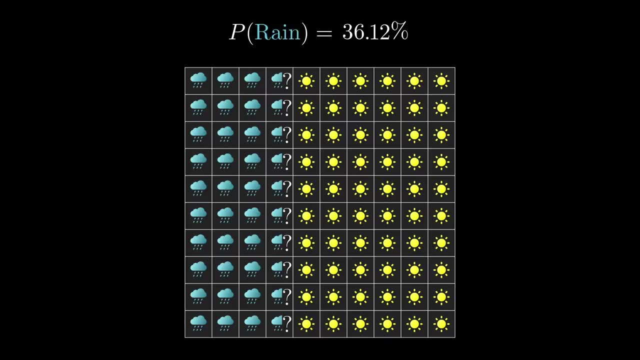 abstractly referencing the idea of something being more or less likely. That said, representative samples don't easily capture the continuous nature of probability. so turning to area is a nice alternative, not just because of the continuity, but also because it's way easier to sketch out. 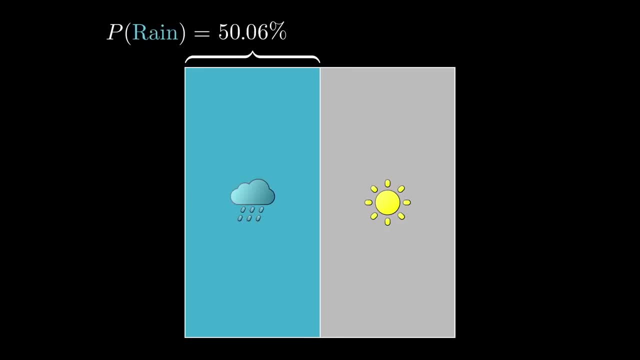 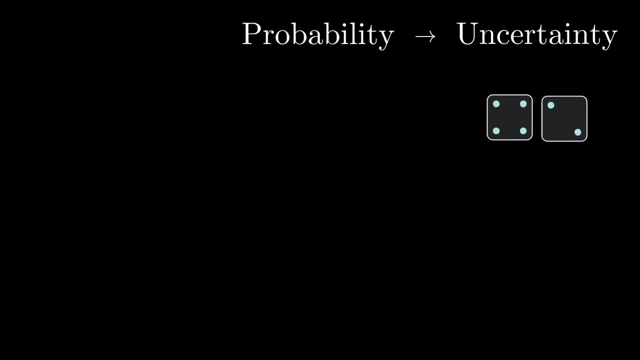 when you're sitting there, pencil and paper, puzzling over some problem. You see, people often think about probability as being the study of uncertainty, and that is, of course, how it's applied in science. but the actual math of probability, where all the formulas come from, is just the 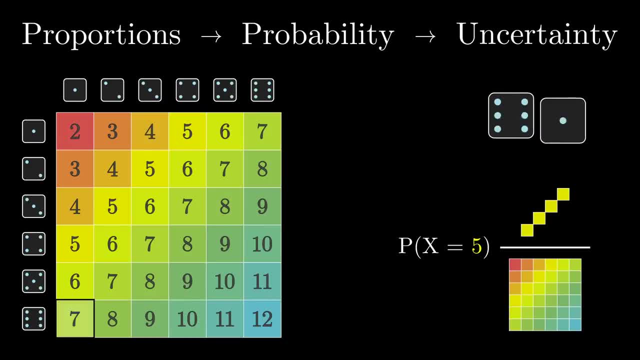 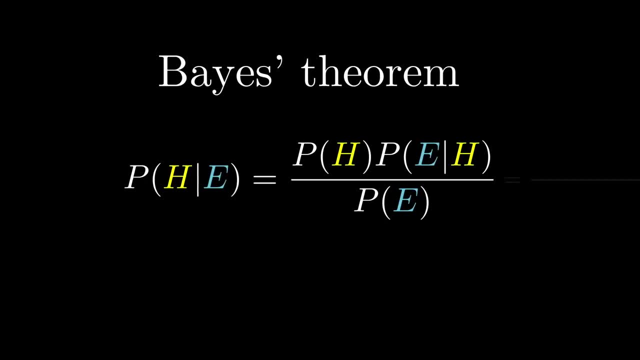 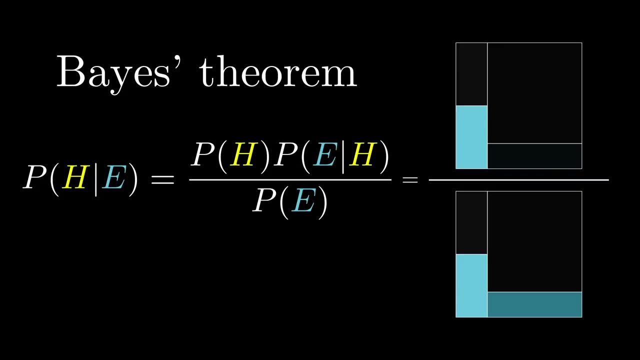 math of proportions and in that context, turning to geometry, is exceedingly helpful. I mean, take a look at Bayes' theorem as a statement about proportions, whether that's proportions of people, of areas, whatever. Once you digest what it's saying, it's actually kind of obvious. Both sides tell you to look at. 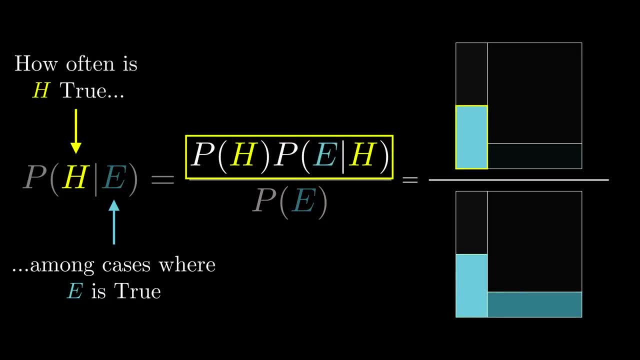 the cases where the evidence is true, and then to consider the proportion of those cases where the hypothesis is also true. That's it. that's all it's saying. the right-hand side just spells out how to compute it. What's noteworthy is that such a straightforward fact about proportions can become 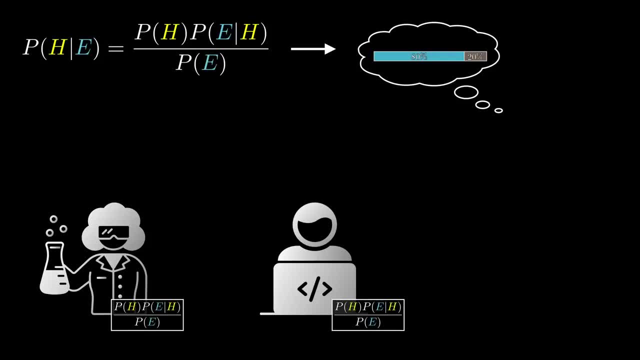 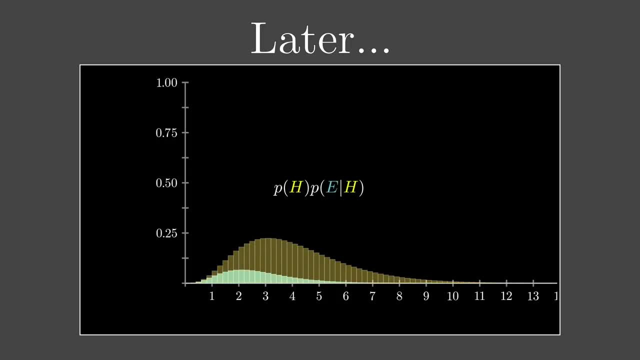 hugely significant for science, for artificial intelligence and really any situation where you're looking to quantify belief. I hope to give you a better glimpse of that as we get into more examples, But before more examples we have a little bit of unfinished business with Steve. 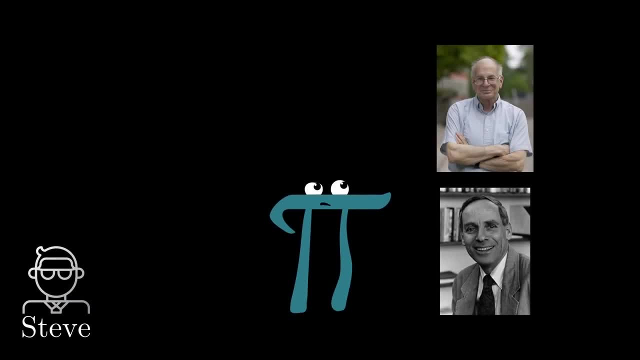 As I mentioned, some psychologists debate Kahneman and Tversky's conclusion that the rational thing to do is to bring to mind the ratio of farmers to librarians. They complain that the context is ambiguous. I mean, who is Steve exactly? Should you expect? 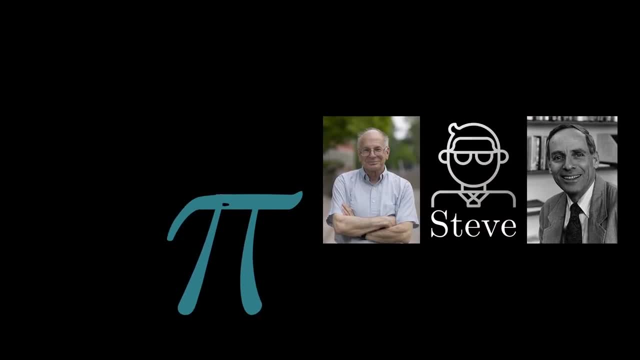 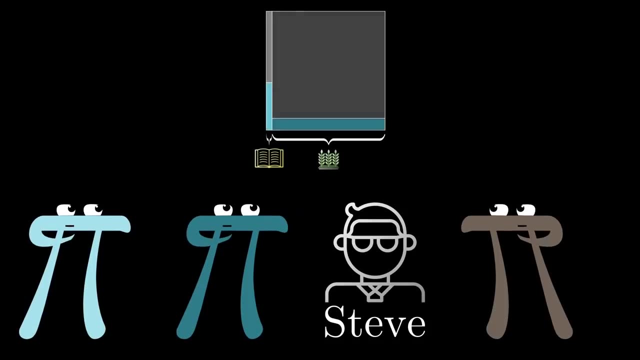 that he's a randomly sampled American, or would you be better to assume that he's a friend of the two psychologists interrogating you? Or maybe that he's someone you're personally likely to know? This assumption determines the prior. I, for one, run into way more librarians in a given month than 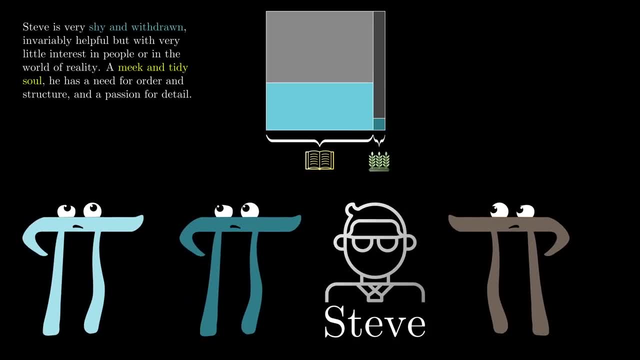 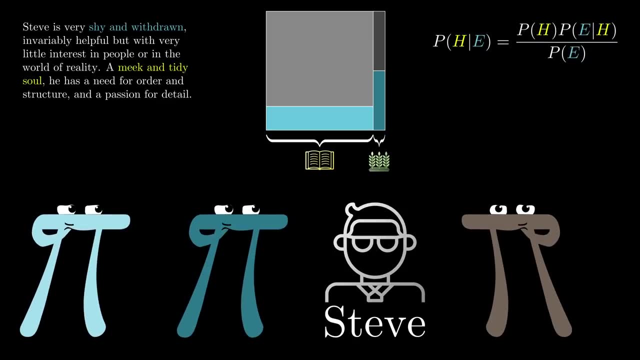 I do farmers And needless to say, the probability of a librarian or farmer fitting with this traction or description is on a highly open level For our purposes understanding math. I emphasize that any important question here can be Christ and realistically added different to the context and can typically be Why? because it's typical for którzy to wag their tail and talk aboutprochen questions like that. Questions about the context shift around the prior in one chit-chat, but commonly the hypothesis often graphing an analogy. Questions about the context shift around the prior. In the beginning. the students understand the.